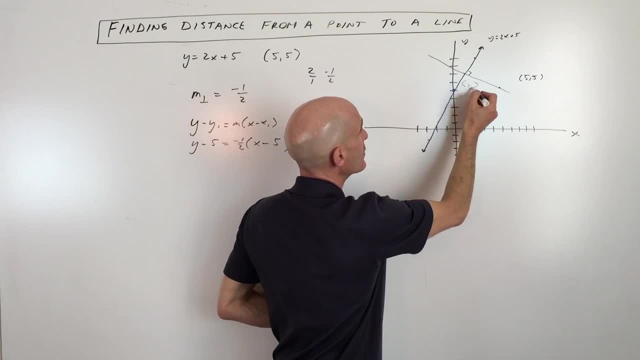 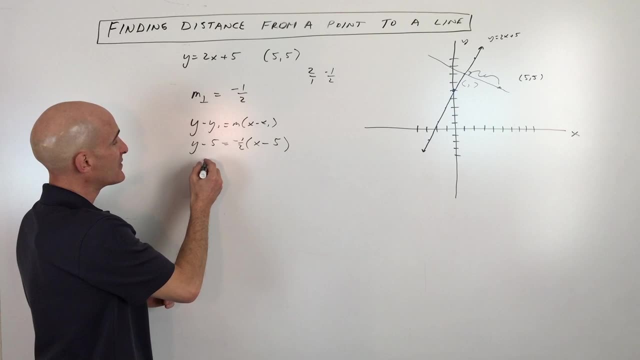 out where these two lines cross. We're going to find the coordinates of this point right here. Then what we can do is we can use the distance formula to find that distance. So let's go ahead and do that. So I'm going to simplify this equation a little bit more for us by 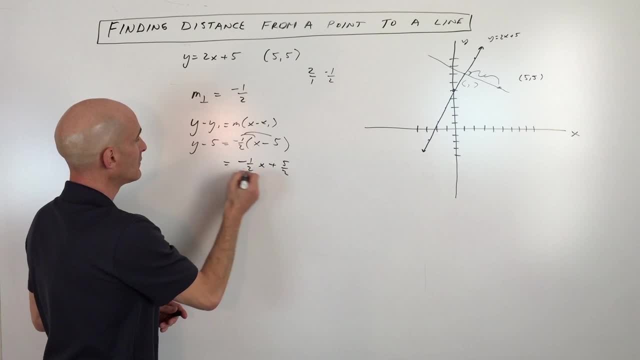 distributing the negative one half, Then I'm going to add 5 to the other side. So that's y equals negative one half, x Add 5.. So 5 is really like 10 over 2. So that's going to be plus 15 over 2. And 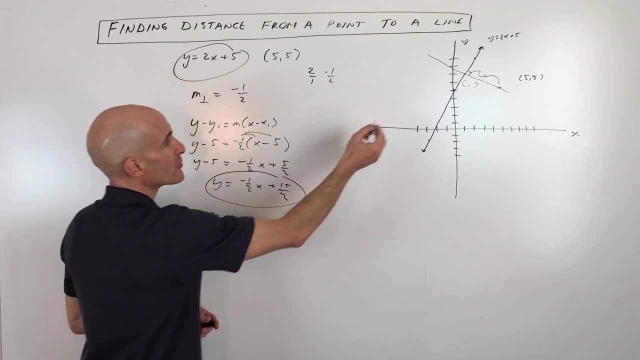 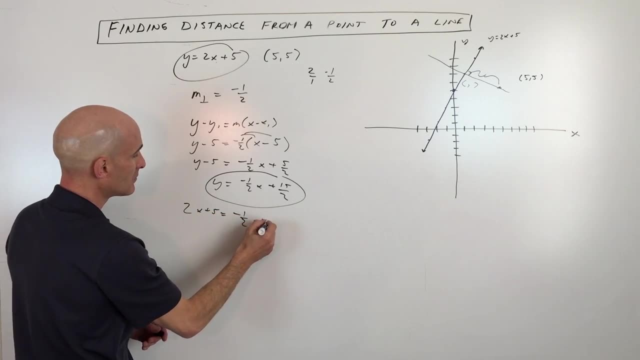 now we have our two equations. I'm going to set them equal to each other to find that point of intersection. So I'm going to put 2x plus 5 in for y here, And then what we're going to do is we're going to 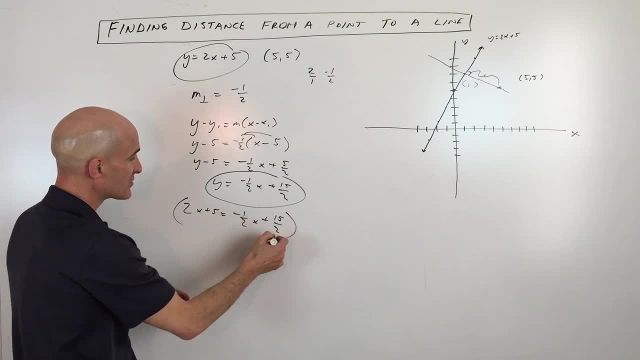 multiply through by 2, just to clear the denominator. So if I multiply everything in this equation times 2, we get 4x plus 10 equals negative x plus 15.. Now that'll make it a little bit easier to solve. So if I add x to both sides, that's going to be 5x. If I subtract 10 from both. 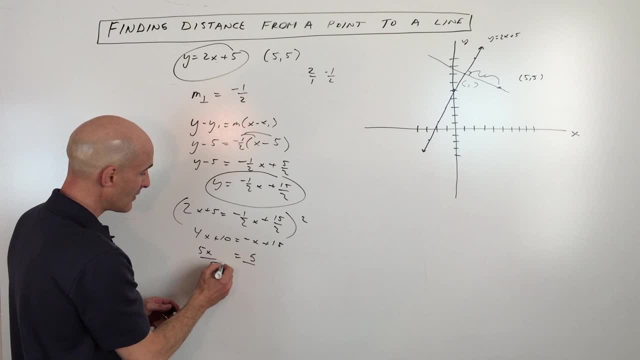 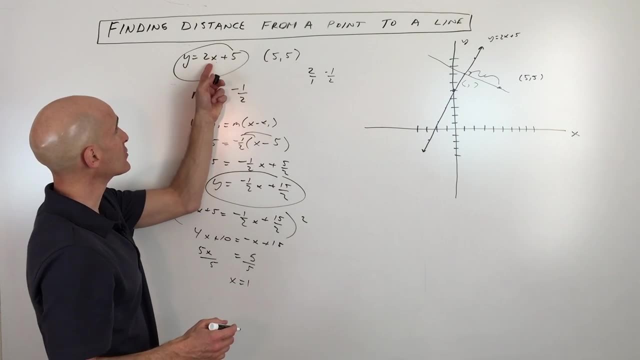 sides, that's going to be 5.. And if I divide by 5, you can see that x equals 1.. Now if I put 1 back in to either equation, I'll just put it into this equation here- 2 times 1 is 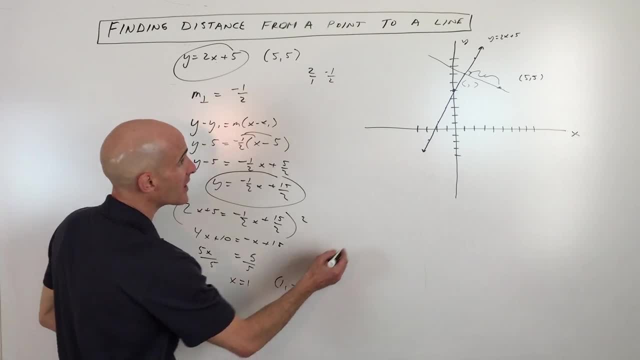 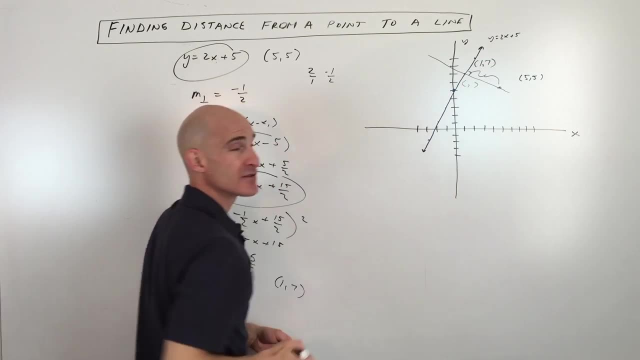 2 plus 5 is 7.. So you can see that these points are going to cross here at 1 comma 7.. 1, 7.. Now all we have to do is find the distance from 1, 7 to 5, 5.. And we've got it. So just a refresher. the 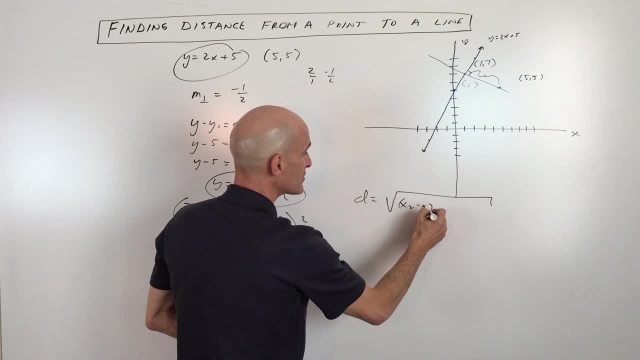 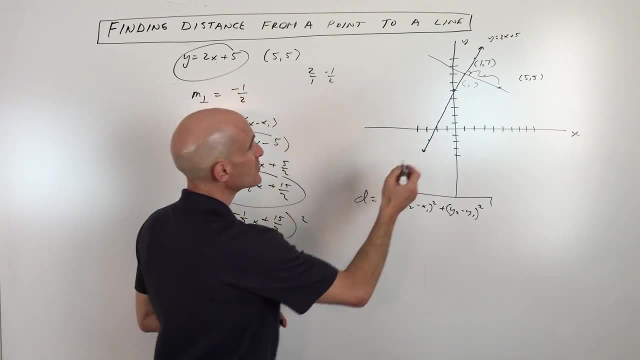 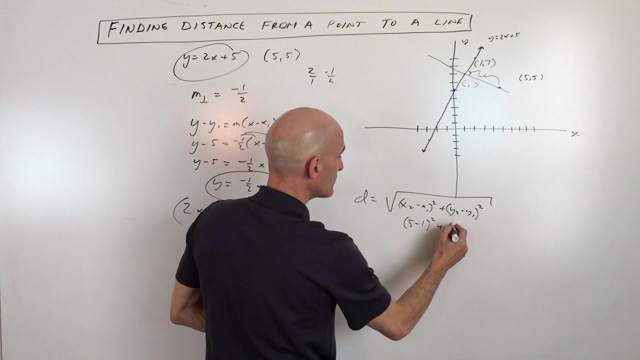 distance formula is the square root of x2 minus x1 squared plus y2 minus y1, the quantity squared And you take the square root of that. So in this case we've got, Let's see, 5 minus 1 squared plus 5 minus 7 squared. Add those together and take the square. 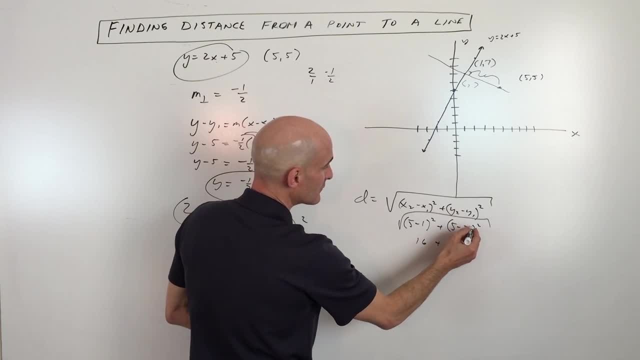 root. So that's 4 squared, which is 16, negative 2 squared, which is 4.. This is the square root of 20.. Square root of 20 is 4 times 5.. Square root of 4 is 2.. So this is going to be 2 square root of. 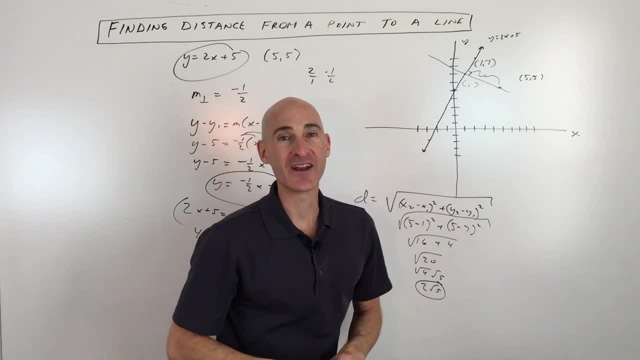 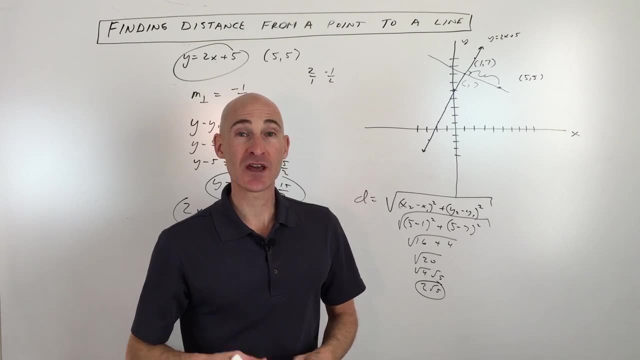 5. So that's the shortest distance from the point to the line, So I hope this helped you to understand how to work through these problems a little bit better. Subscribe to the channel. Check out more math tutoring videos on Mario's Math Tutoring. 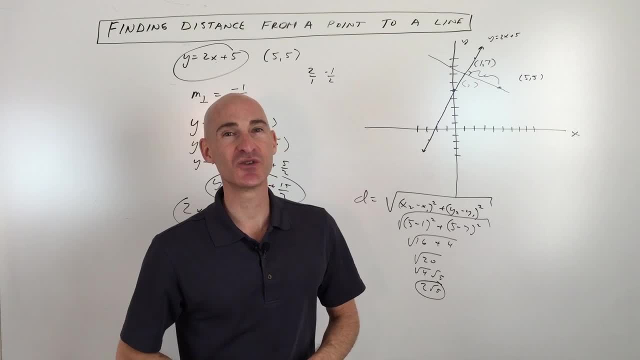 YouTube channel And I look forward to helping you in the future videos. I'll talk to you soon.